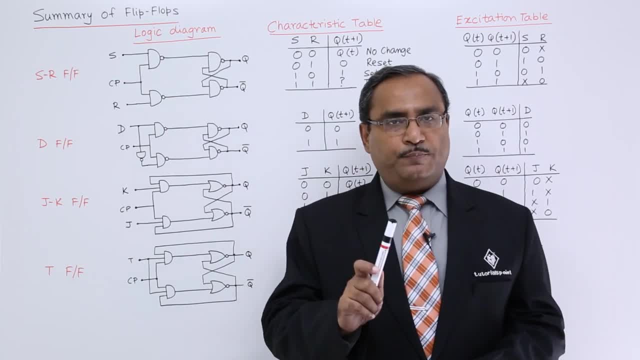 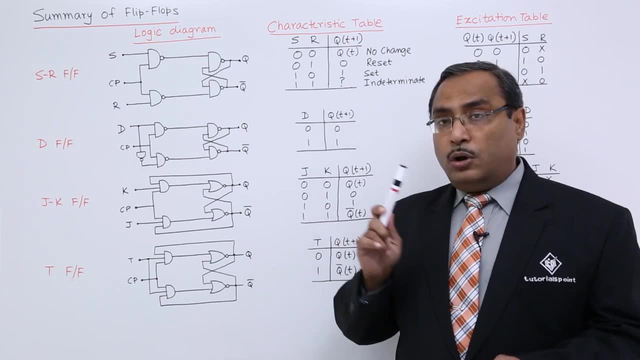 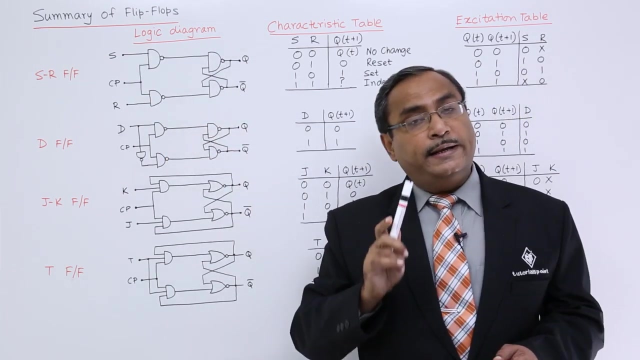 SR flip-flop. SR stands for set reset flip-flop. So this is the circuit for the SR flip-flop. We discuss about the details in the respective video. Always remember: whenever in the clock logic we are having NAND, then in the flip-flop logic we will be having NAND Whenever the 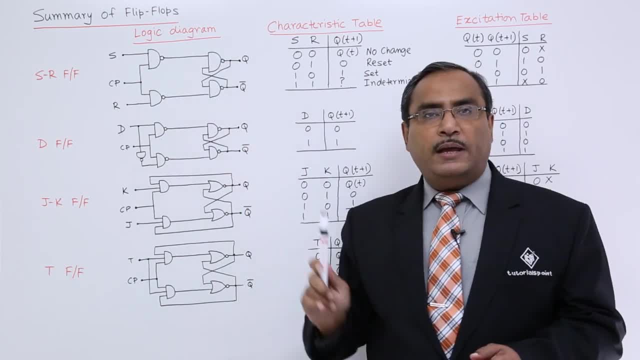 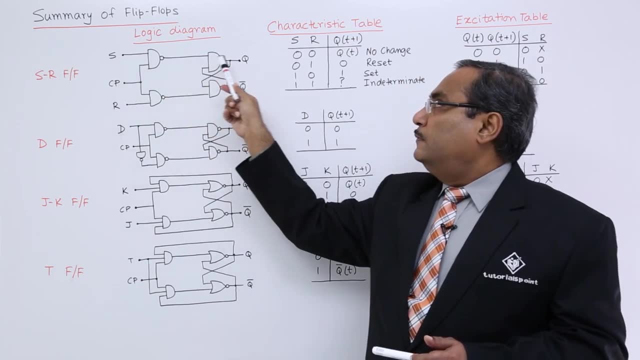 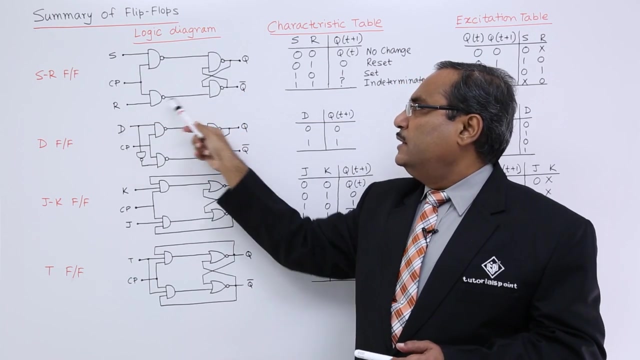 clock logic is having, AND then the flip-flop logic will be having NOR. Whenever NAND logic is there, then S will have NAND. So in the same way, if S is there, then Q will be there. If you mark this one, S, then 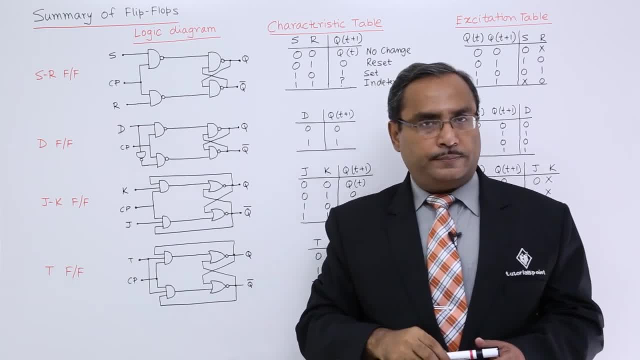 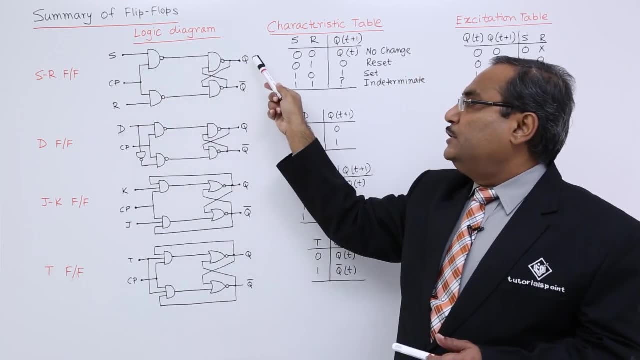 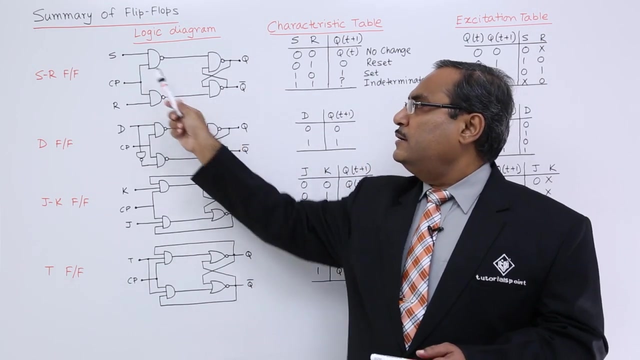 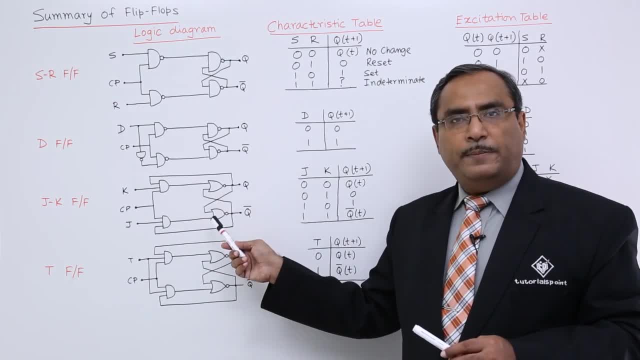 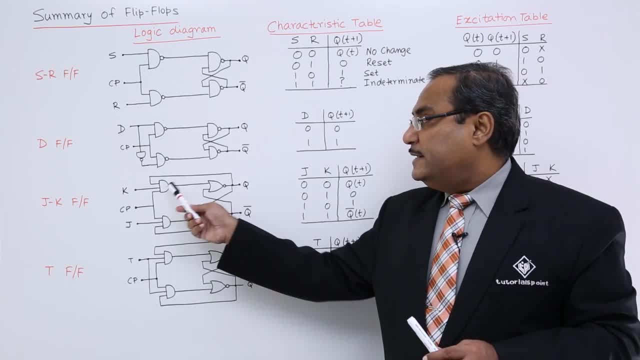 will be facing Q. So then K will be facing Q. If it is NAND-NOR, logic is having AND FIP-LOP logic will be having NOR CLOCK logic is having NAND, then FIP-LOP logic will be having NAND. If it is NAND-NOR logic, then K will be facing. 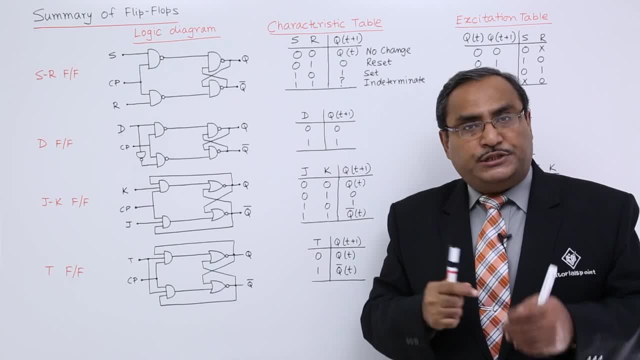 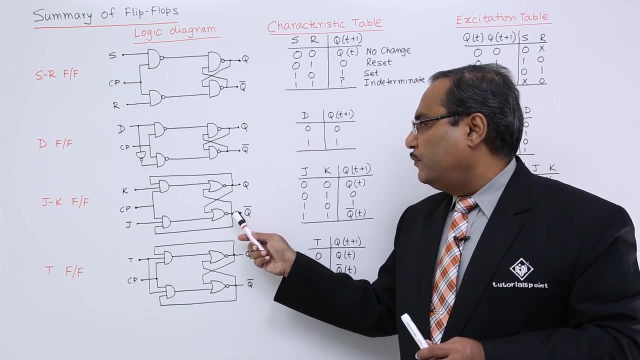 Q and in case of NAND-NAND logic, then K will be facing Q And another change will take place. That means Q will be going here and Q-BAR will be coming here, but the feedback path to K will be going for Q only. so the path will be something like this: 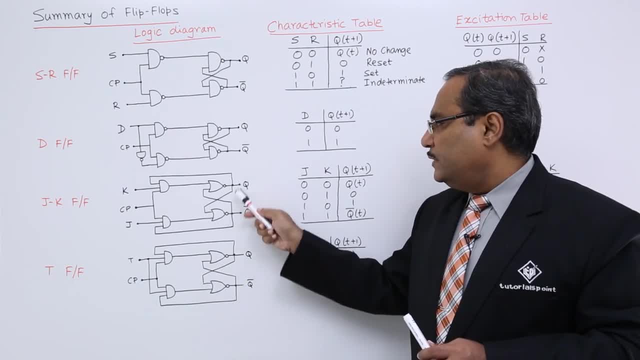 So now you come to the next step. if you, if you take the input, you will get the input. So, here, this path will be taken from there and this path will be taken from there. So there will be a crossover. 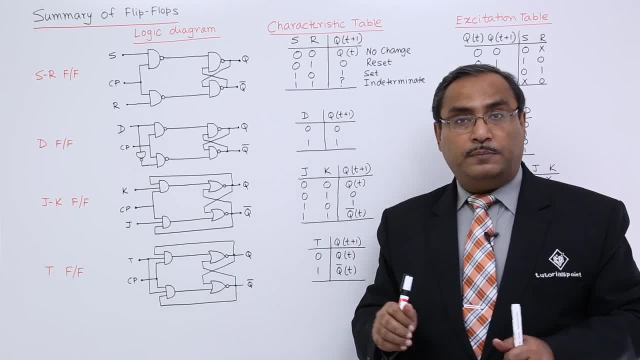 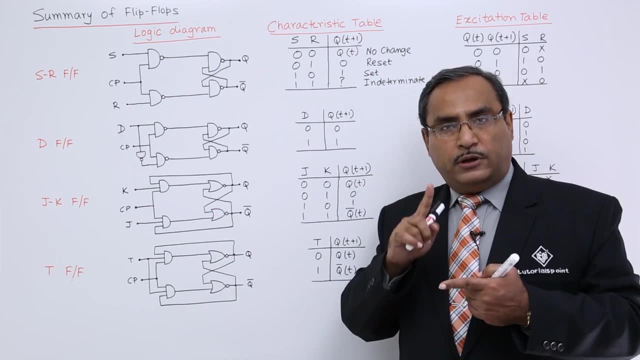 So in this way that is a case for the JK flip-flop using two different circuits. Now, in case of JK flip-flop it is a 2 bit flip-flop because j and k 2 bits are there. So 4 input combinations can be possible and it is free from rest condition. 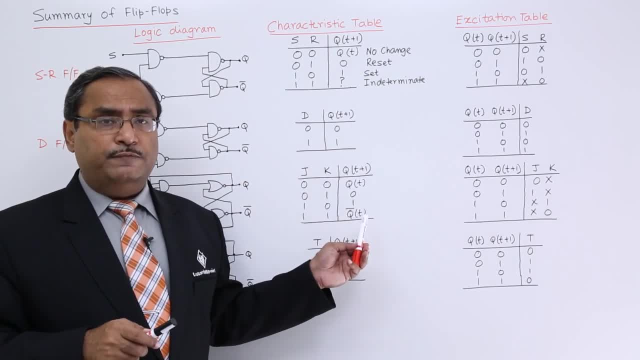 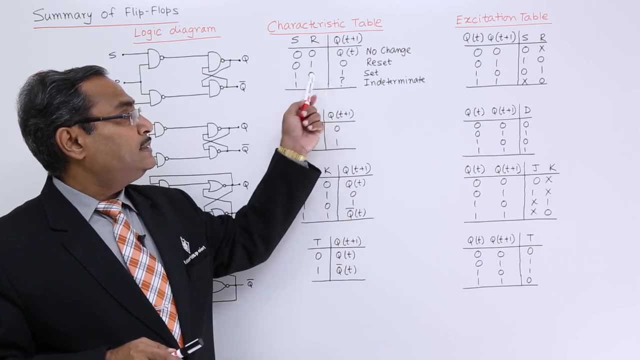 So here is a respective characteristic table for JK flip-flop. So for 0: 0 it is q, t, for 0: 1 it is 0, for 1: 0 it is 1. same as the SR flip-flop, but for: 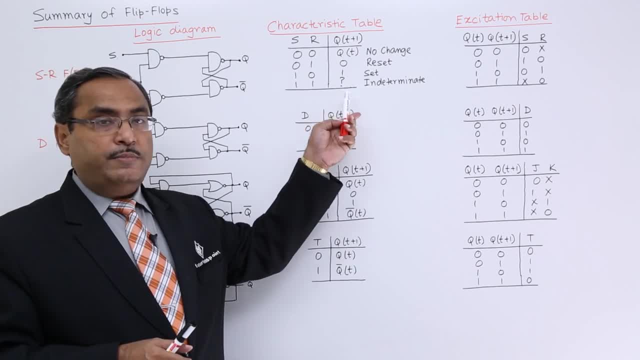 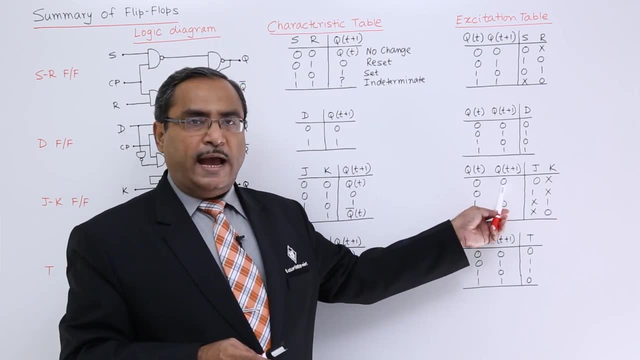 1. 1 it is q bar t, So here it was indeterminate part. it is q bar t. So 0 to 0 we can consider in two ways. that means no change and set, no change and reset, because 0 is there. no change and reset. 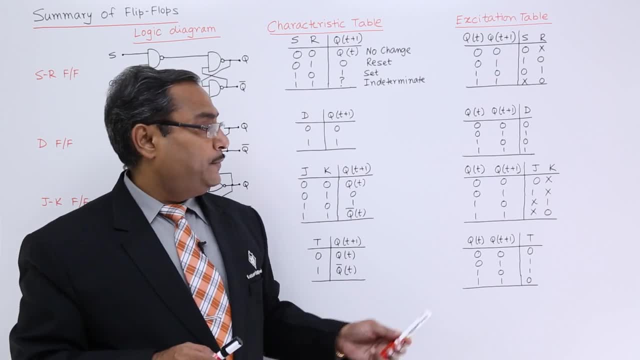 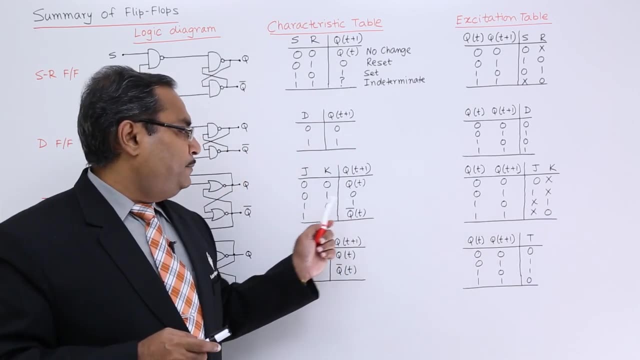 So input should be 0- x. as I explained earlier, 0 to 1 can be thought in two different ways. What is that? That is set? set means input should be 1- 0 or output is getting complemented. input should: 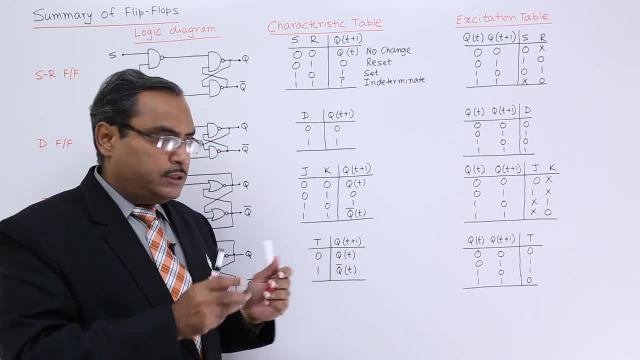 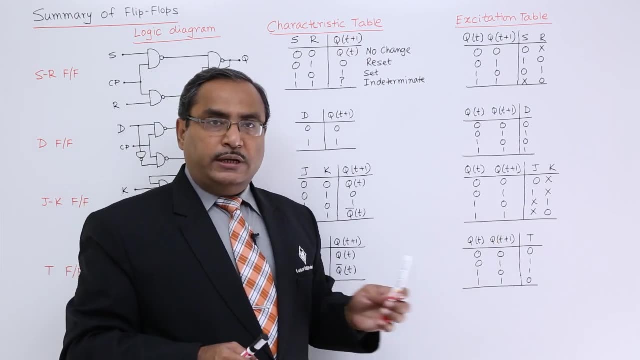 be 1- 1.. So 1: 0 and 1: 1. if you merge, then you are getting 1 and x. so you are getting 1 and x there. From 1 to 0 transition can be thought of in two different ways. either the output is getting: 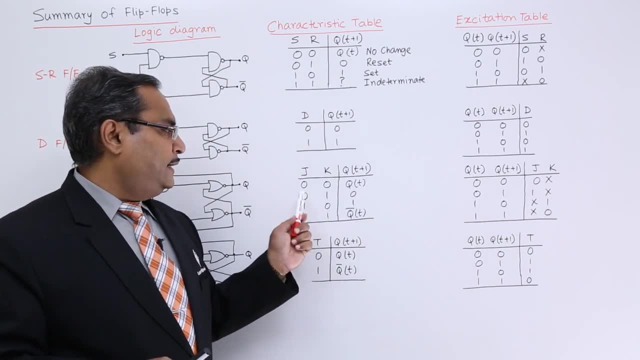 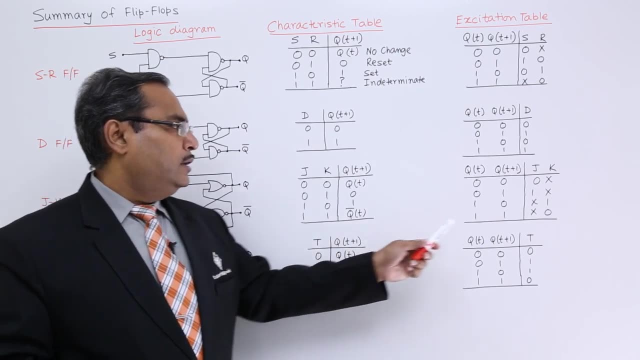 reset or output is getting complemented. For reset, input should be 0: 1, output should be complemented. So if you merge them, it is x: 1, so that is why x: 1 and 1: 1 can be thought of in two different. 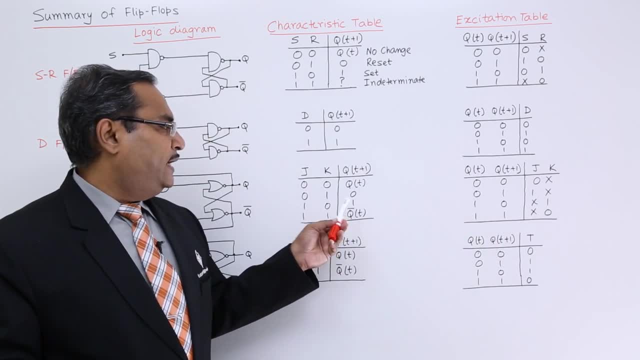 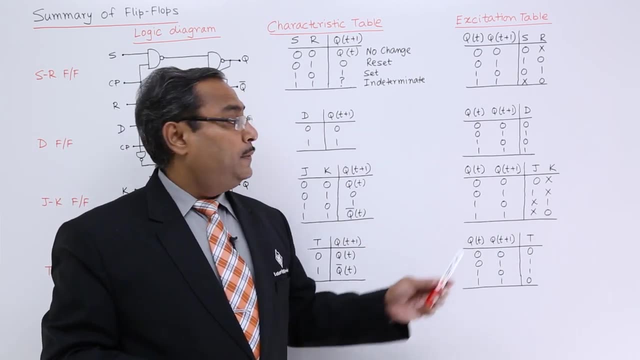 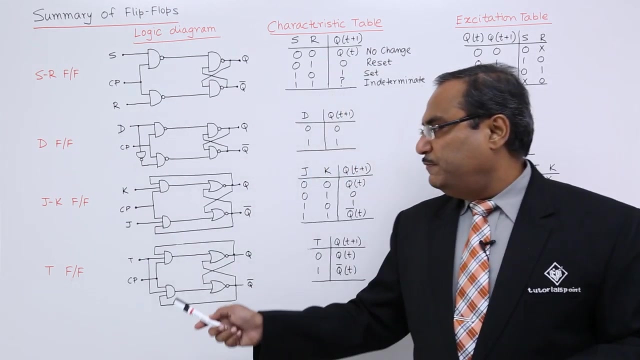 ways. either it is set or no change. So set means this one, no change means this one. if you merge them, it is x: 0.. So that is our JK flip-flop. that is the x addition table here. Next we are going for the last one, that is our T flip-flop. in case of T flip-flop, the 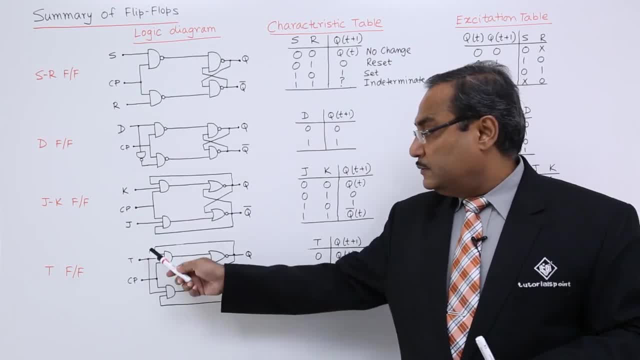 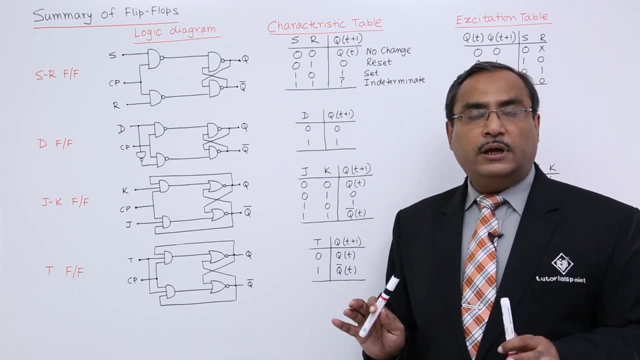 J and K terminal is getting shorted by 1: 0.. By shorted by a simple wave. so that is why they are getting directly shorted. and here is the clock pulse. and here is the circuit diagram for the T flip-flop. 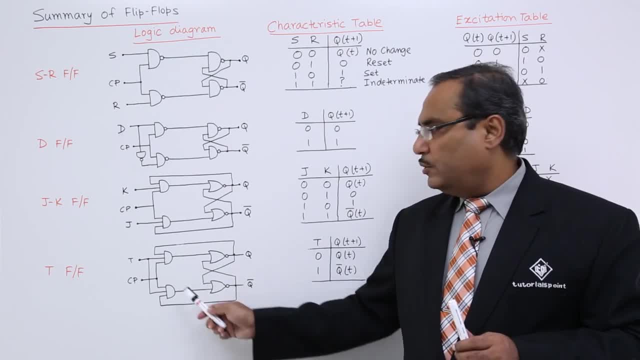 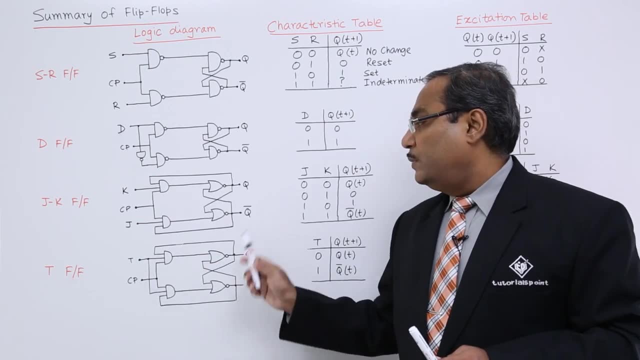 And similarly here: if the logic is AND, the flip-flop logic will be NOT, if the clock logic is NAND, flip-flop logic will be NAND in the case, and here T will be facing Q. but at that time T will be facing Q. but in this way you can think. but actually the thing, 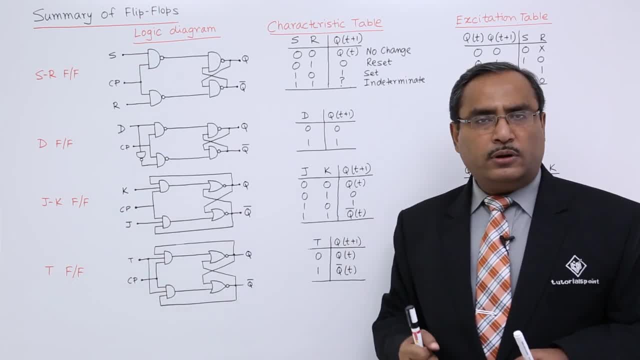 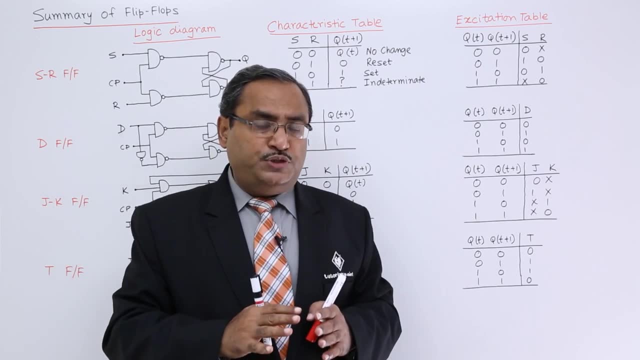 is that also. you can consider this one as T, you can consider that one also as T, because both are getting shorted. So that is our T flip-flop. So T flip-flop means a special case of JK flip-flop. where T is equal to 0 means JK is. 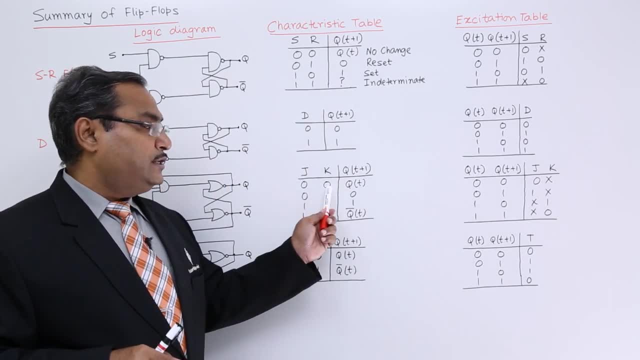 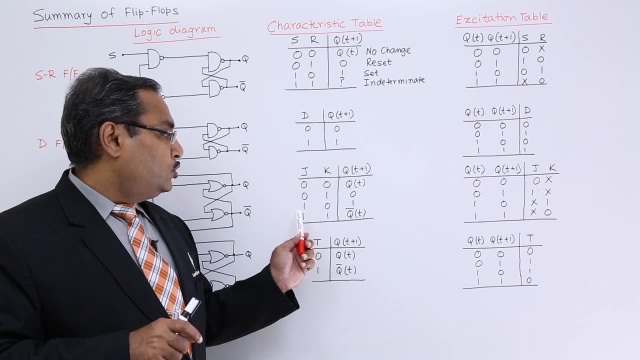 equal to 0: 0.. So that means T 0 means JK: 0: 0.. So Q: T will be the output and T 1 means JK, the in case of JK it is 1: 1.. So T 1 means JK is 1: 1, so that is, we are having this Q but T here. 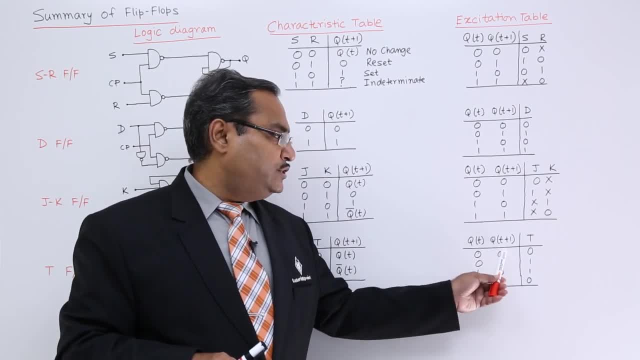 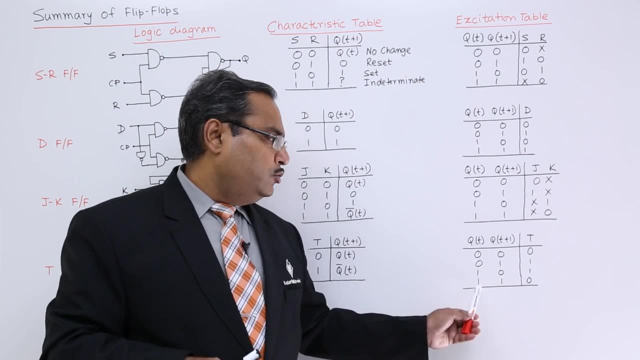 So now, if we want to change in the output, do you want to change in the output? No, input should be 0,. do we require the change in the output? Yes, input should be 1,. do we require change in the output? 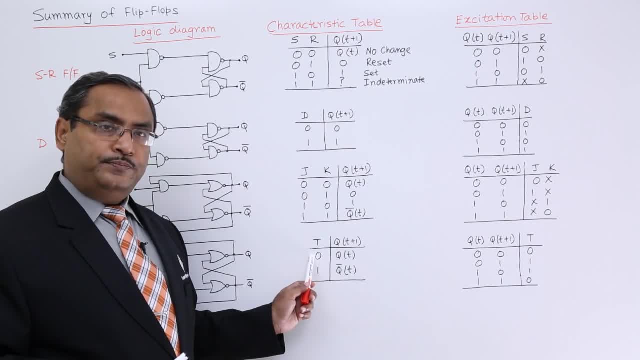 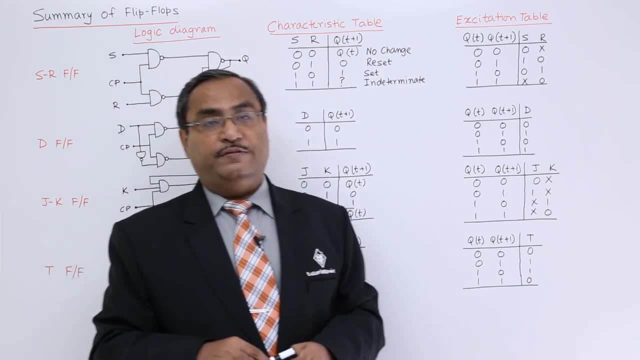 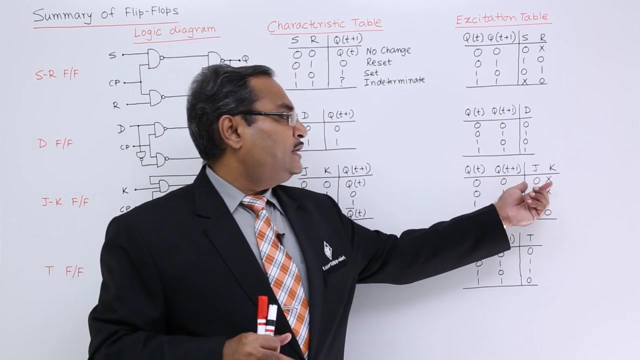 No input should be 0.. So when input is 0,, then there is no change in output. when the input is 1, there is a change in the output, And that is the logic of T flip-flop. In case of circuit design, sequential circuit design, we remember the sequence that is 0x1xx1x0,. 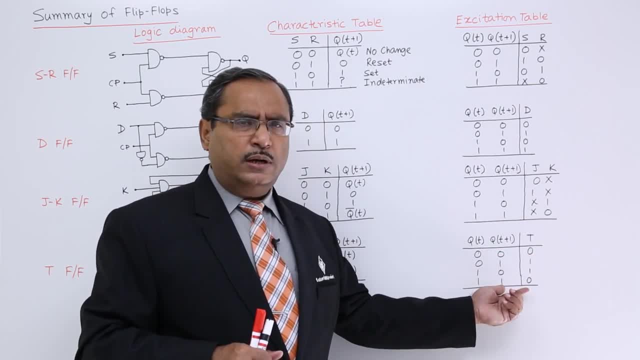 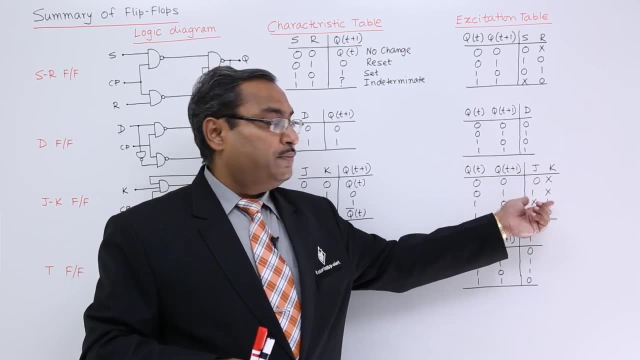 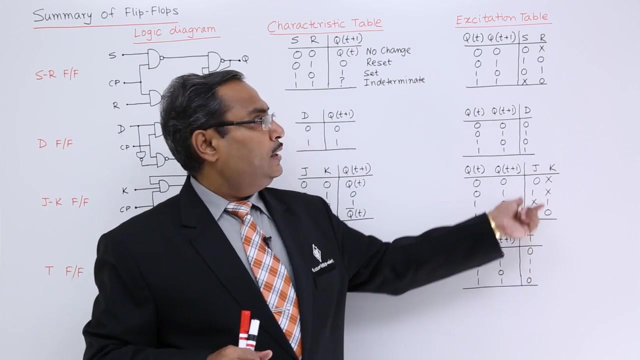 if you can remember this one, this particular x addition tables are very simple. for d and t they are very simple, but just remember the respective sequence for the j, k, x addition table. So it is 0 x, 1 x x, 1 x 0. if you can remember this one. it is very simple. it is 0 x, it is not 1, 0 it. 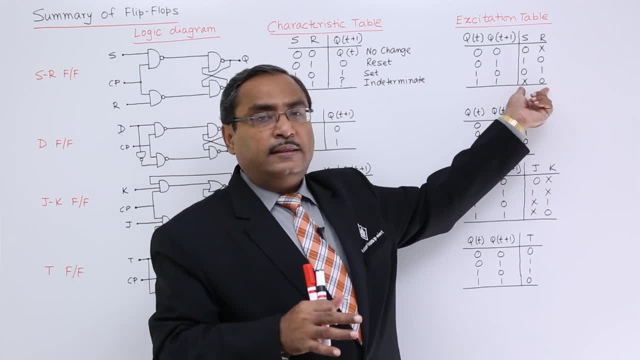 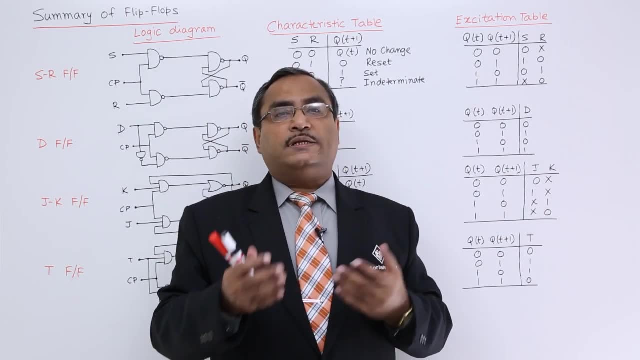 is not 1 x, it is 1: 0, then it is 0: 1 and this is my x: 0.. So that is why in the exam one question may come: that j k flip-flop is more flexible than s r flip-flop. how to answer? 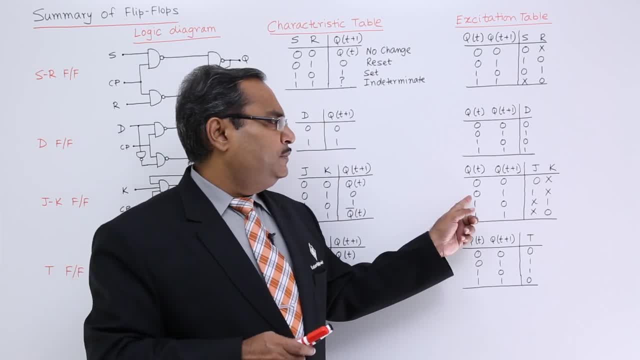 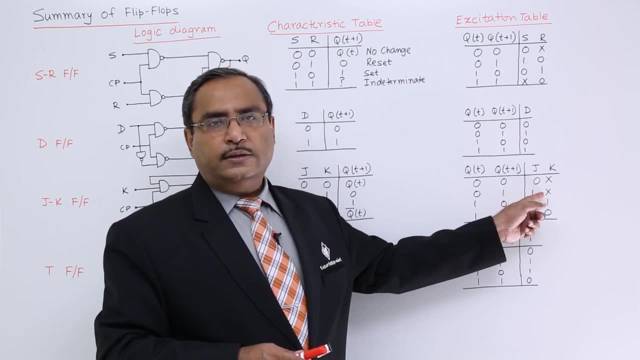 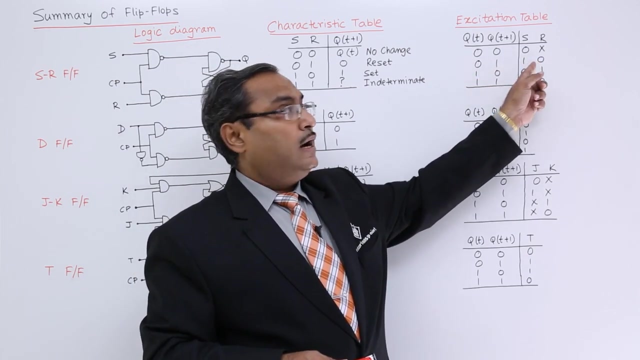 this one. You can answer this one in this way that in case of 0 to 1 transition, in case of j- k flip-flop, I require to have 1 in j, but anything is allowed in k, but in case of 0 to 1 transition, we require 1 in s and 0 in r for 1 to 0 transition. 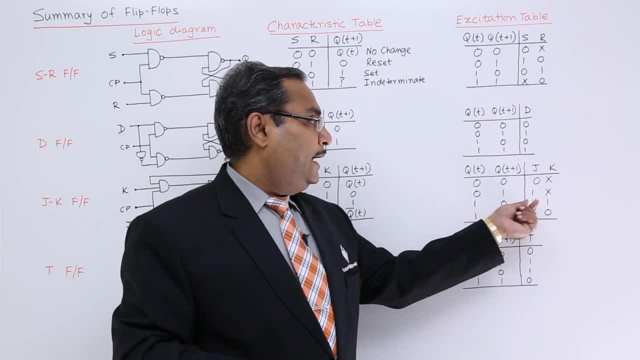 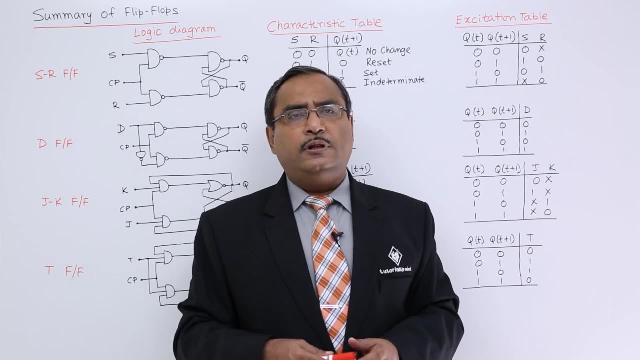 I require 0 in s and 1 in r, but here anything in j and 0 in r. So that is another answer to prove that j k flip-flop is flexible than s r flip-flop. So please remember the sequence. that is 0 x, 1 x x, 1 x 0. similarly, you can have this: 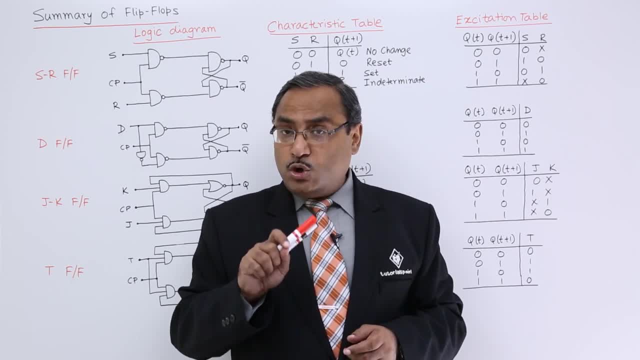 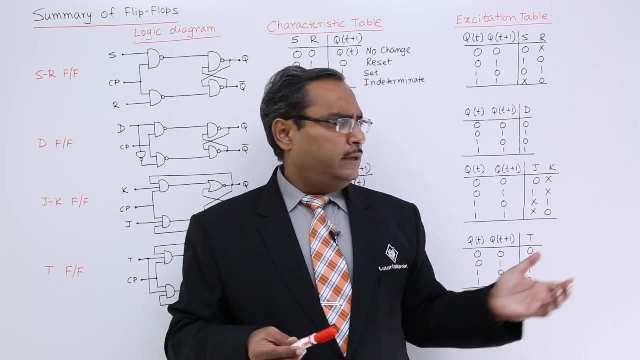 one as 0, x, 1, 0, 0, 1 and x 0.. So that is, this is the respective excitation table for s r flip-flop. other excitation tables are quite simple. you can easily get it as one to recall.